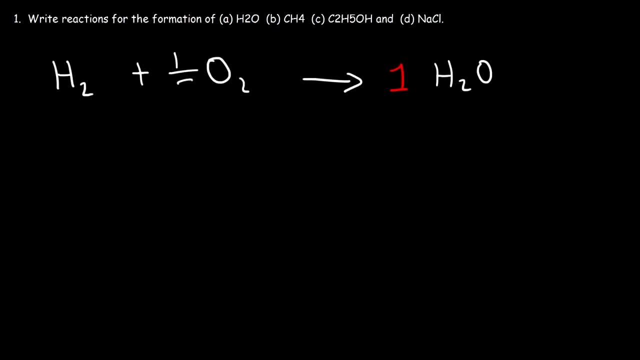 Now, to balance it, we need to put a one-half in front of O2, because we only have one oxygen atom on the right side, And so that's how you can write the formation reaction for water. Now go ahead and try it with methane. So keep in mind whenever you're writing the formation of a. 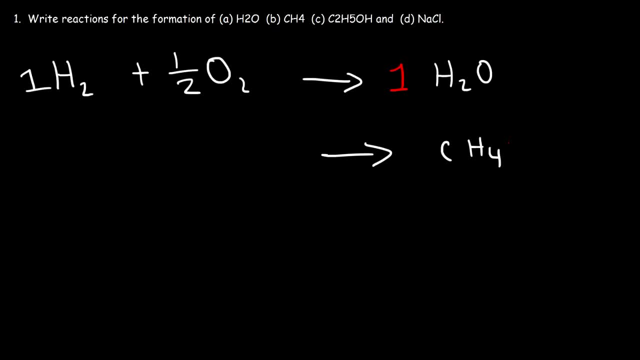 substance, you need to have one mole of that substance on the right side of the equation, So make sure the coefficient is one. So methane contains carbon and hydrogen. So carbon naturally is a solid and hydrogen is a gas, And all we need to do and notice the balance is to write the 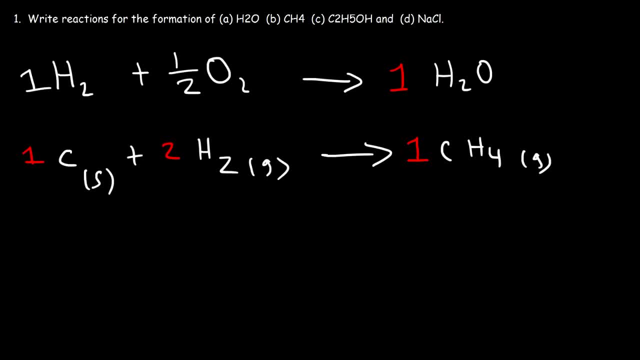 factor of one in front of O2.. Hence we need to put it two in front of H2, And so that's it. This is going to be a liquid, and these two are gases. Now what about this one? Part C: 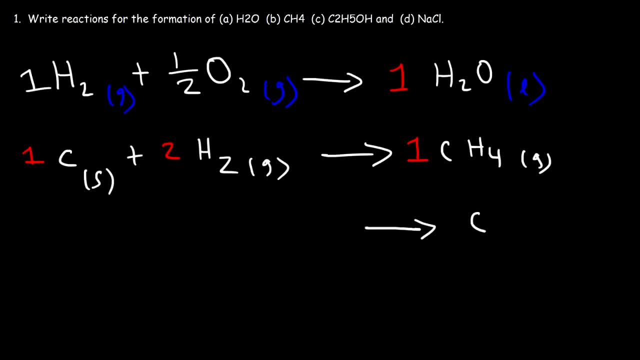 Write the formation reaction for ethanol. So ethanol consists of carbon, It consists of hydrogen gas. So it can be a reaction to water, but we don't know if it's a reaction to carbon. So let's just write that out right at the very end. So the reaction- reaction for hydrogen- is called reaction to water. 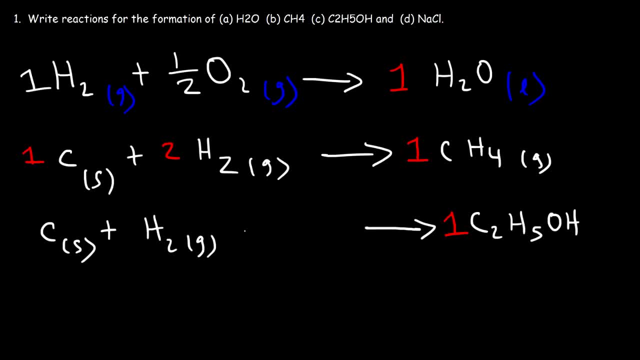 and we also need oxygen gas to make it, and ethanol in its natural state is a liquid at room temperature, so we need to balance it. we got two carbon atoms on the right side. we have a total of six hydrogen atoms on the right, so we need to put a three in front of h2 and we 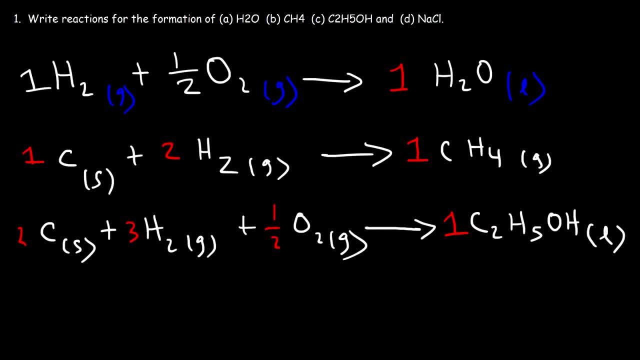 only have one oxygen atom on the right side, so we need a half in front of o2, and now it's balanced. now for the last one. we simply have sodium chloride, which is a solid at room temperature, and it's composed of sodium, metal and chlorine gas. so to balance it we need a one-half. 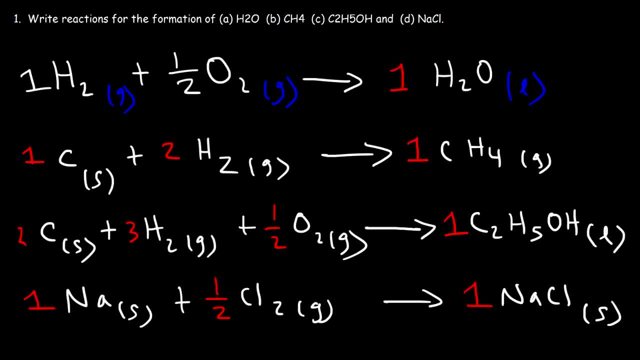 in front of cl2, and so that's how you can write the formation reactions for substances such as those. ok, now you need to understand that the enthalpy change for this reaction is equal to the enthalpy of formation of water. if you look at the appendix in your 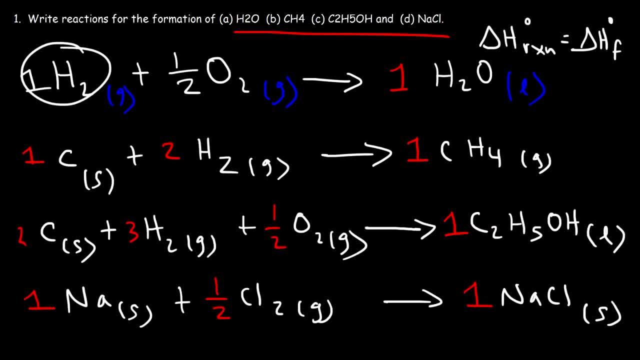 chemistry textbook, you'll see that the heat of formation for any element in its natural state is going to be zero. therefore, the enthalpy change for the reaction is equal to the heat of formation of this compound. the same is true for all of them: carbon hydrogen gas. 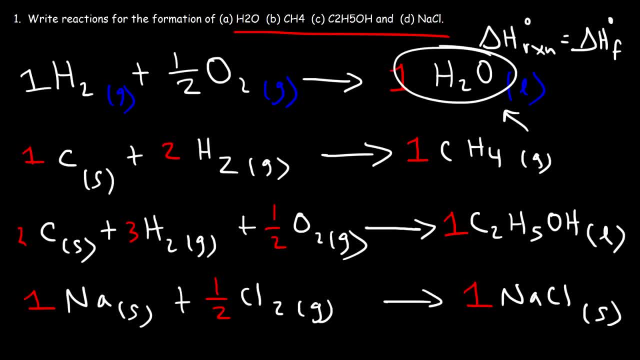 oxygen gas. they all have a heat of formation of zero. so therefore, for each of these reactions, the spp of the reaction is simply equal to the heat of formation of the product. now let's move on to this example right of reaction, for which the enthalpy 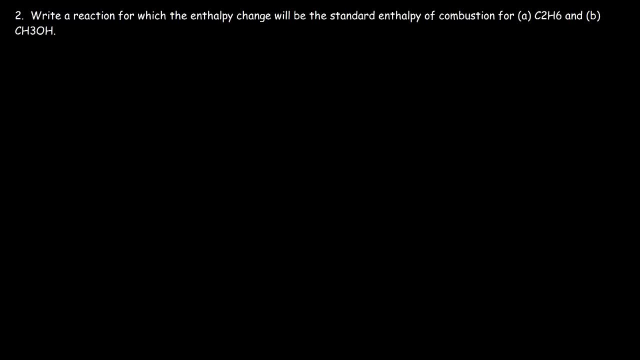 change will be the standard and to be a combustion for ethane and methanol. so all you need to do for a problem like this is you simply need to write the combustion reaction for each of these substances, so starting with ethane, if you want to write a combustion reaction, 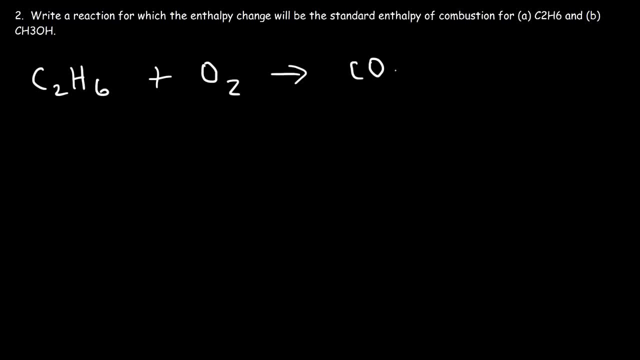 add O2 to the left side and the products will always be the same: CO2 and water. and then you got to balance it, so you need to put a 2 in front of CO2 to make sure the number of carbon atoms is the same. now we have 6 hydrogen atoms on the. 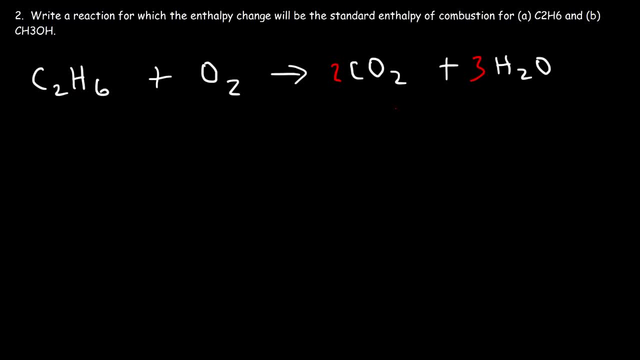 left. so we gotta put a 3 in front of H2O. so this gives us a total of 7 oxygen atoms. 2 times 2 is 4, 3 times 1 is 3. so in order to balance it we need to put a. 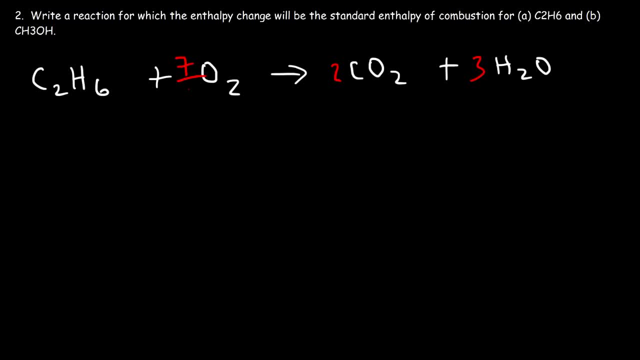 fraction on the left side. so this is going to be 7 over 2 for oxygen. so this reaction is going to be equal to the enthalpy of combustion for ethane C2H6. so make sure you understand that the enthalpy change of 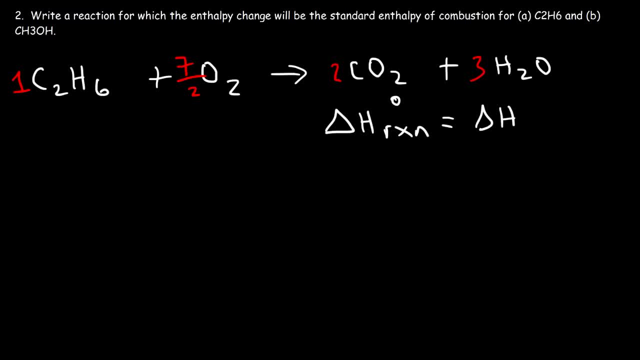 this reaction is simply equal to the enthalpy of combustion for one mole of ethane. now let's do the same for methanol. so we're going to be active with O2 as well, and whenever you're dealing with combustion, you know you're going to get carbon dioxide and water whenever you have a. 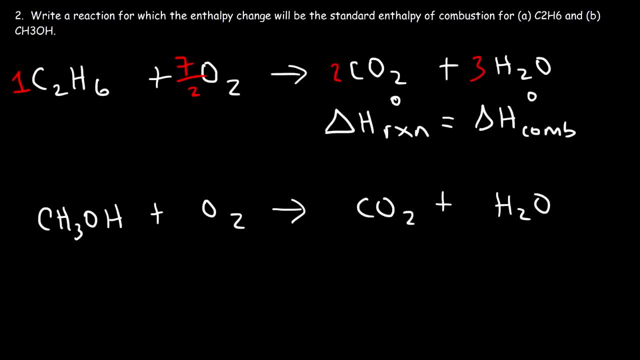 hydrocarbon like this, so the carbon atoms are balanced on both sides. we have one of each. now we have 4 hydrogen atoms on the left, so we got to put a 2 in front of H2O. now we have a total of 4. oxygen atoms are on the right side, and only right now. 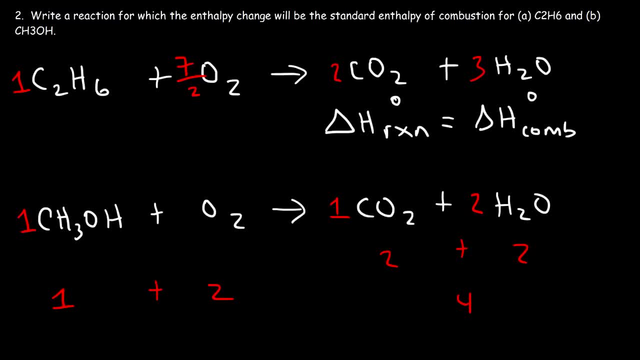 three on the left side and four on the right side. So in order to get 4, we need to make this number 3.. So I'm going to put a 3 over 2 in front of O2.. 3 over 2 times 2, the 2s cancel and you get 3.. So now the reaction is balanced. We have 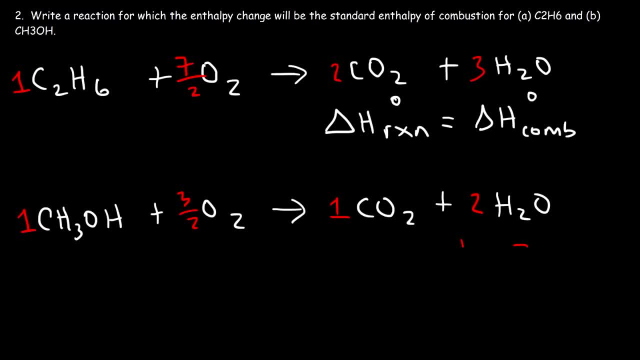 a total of 4 oxygen atoms on both sides. And when dealing with the enthalpy of combustion for this substance, you want to make sure that the coefficient is 1, because you want to find the enthalpy change of the combustion of just 1 mole of methanol and 1 mole of ethane. So the 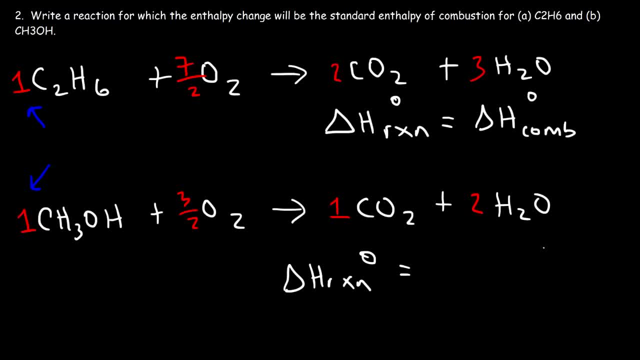 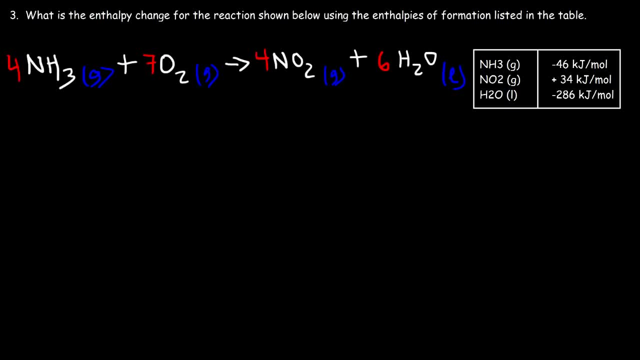 enthalpy of this reaction, as mentioned before, is going to be equivalent to the enthalpy of combustion for 1 mole of methanol. Now, what about this problem? What is the enthalpy change for the reaction shown below using the enthalpies of formation listed in the table? 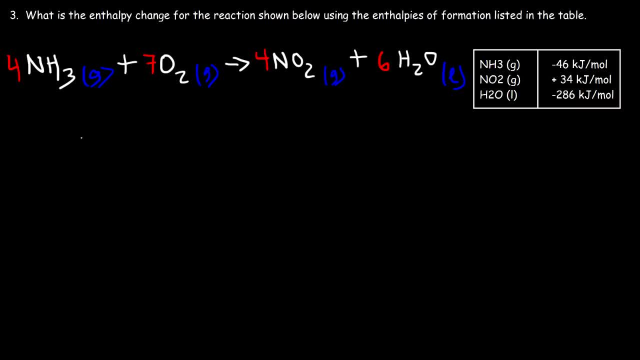 In order to get the enthalpy change for the reaction, we need to find the enthalpy of the reaction. So, in order to calculate the enthalpy change of the reaction, here's the formula that we need to use. It's basically the sum of the heat of formation of all the products. 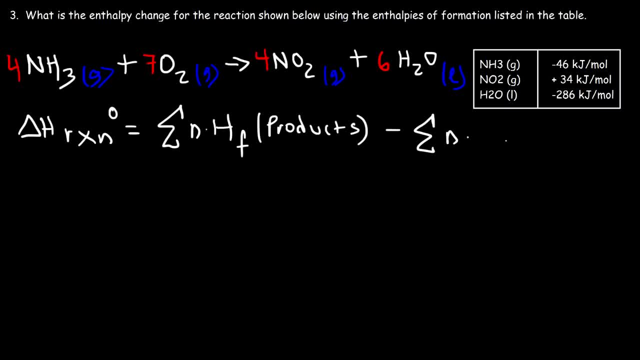 minus the sum of the heat of formation of all the reactants. So perhaps you heard it before, but the enthalpy change of the reaction is going to be equal to the products minus the reactants. If you're wondering what the N stands for, it represents moles In this. 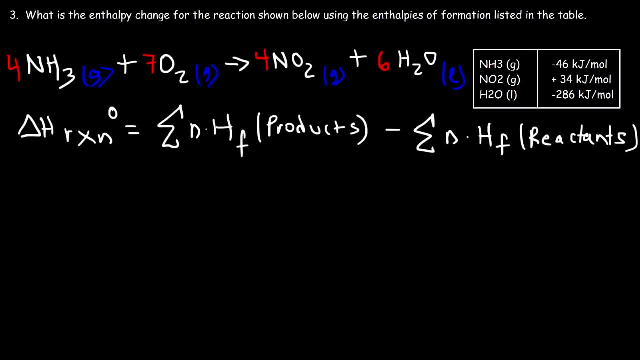 problem. you need to take into account the coefficient in the balanced chemical reaction. So I like to write it this way: The enthalpy change of the reaction is going to equal the products, which are the 4 NO2 molecules and the enthalpy change of the reaction which 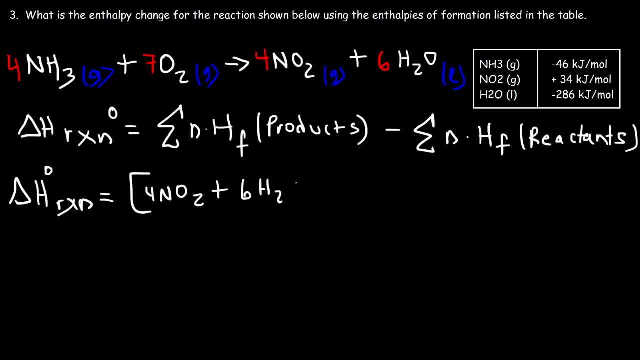 is equal to the 6 water molecules minus the heat of formation of the reactants, which is equal to NH3 and O2.. So at this point, just plug in the numbers that you have. So for NO2, we can see that the heat of formation is 34 kilojoules per mole. So replace NO2. 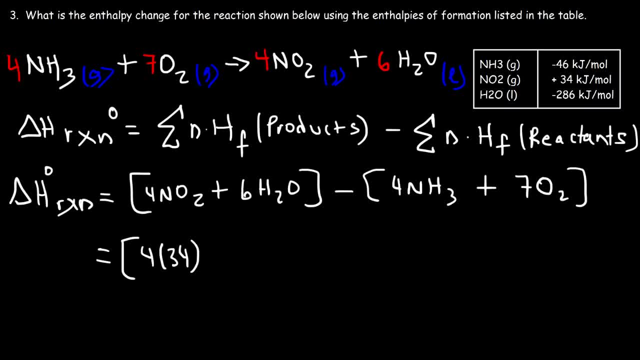 with 34.. But don't forget to multiply it by 4.. And then the value for water is negative, 286,. and then minus for NH3, which is negative 46. Let's multiply that by 4.. Now oxygen is a pure element in its natural standard state, so it's going to be zero for. 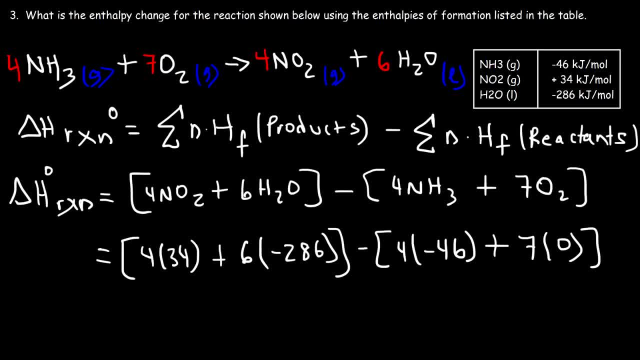 O2.. So the heat of formation for any substance in its natural state- if it's a pure element, by the way- is always zero. So now all you got to do is just type exactly what you see here. So plug these numbers into your calculator and you should get negative 1396 kilojoules. 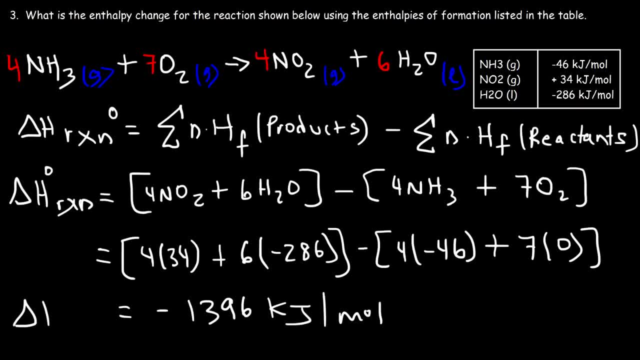 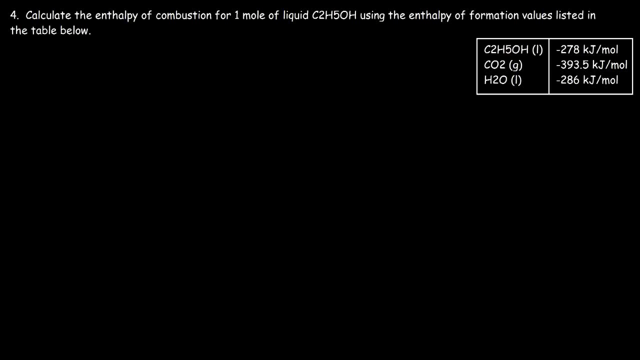 per mole. So that's the enthalpy change. That's the enthalpy change of the reaction listed above. So this is the answer Number 4.. Calculate the enthalpy of combustion for one mole of liquid ethanol using the enthalpy. 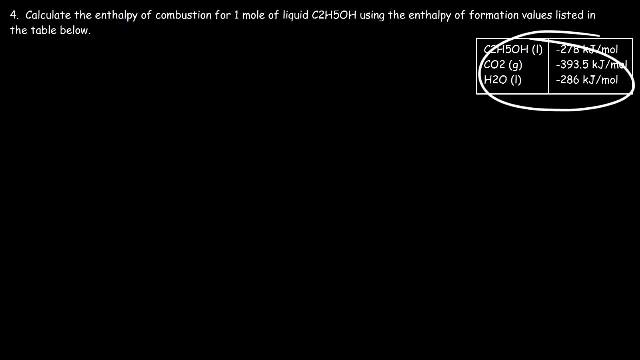 of formation values listed in the table below. So first we got to write the reaction that corresponds to the combustion of C2H5OH, So we did an example like this earlier. All we need to do is react it with oxygen and we know it's going to produce carbon dioxide. 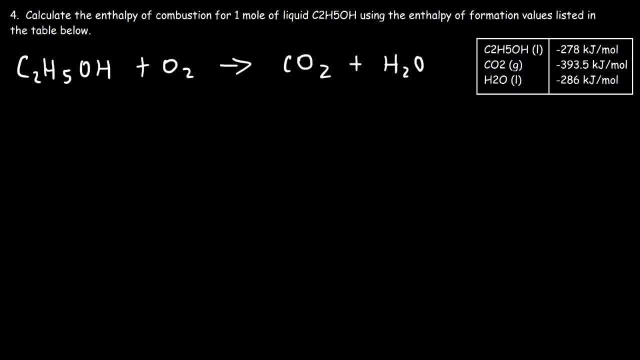 and H2O. Now ethanol is in its liquid state. O2 is a gas, carbon dioxide is a gas and water, in this example, will be used as a liquid. So let's balance the reaction. We need to put a 2 in front of CO2.. 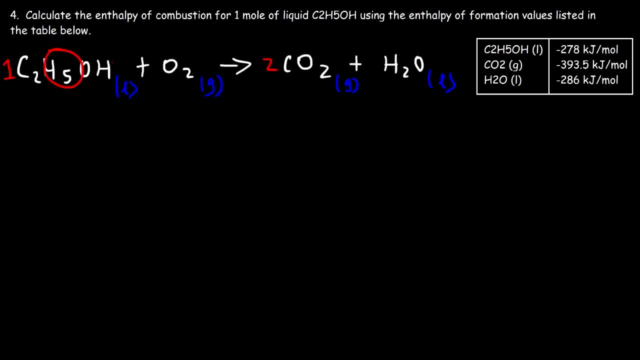 So we can have 2 carbon atoms on both sides. We have a total of 6 hydrogen atoms on the left, so we need to put a 3 in front of water. So now we have 7 oxygen atoms on the right. We already have 1 within ethanol, so we need 6 from O2, so we're going to put a 3 in front. 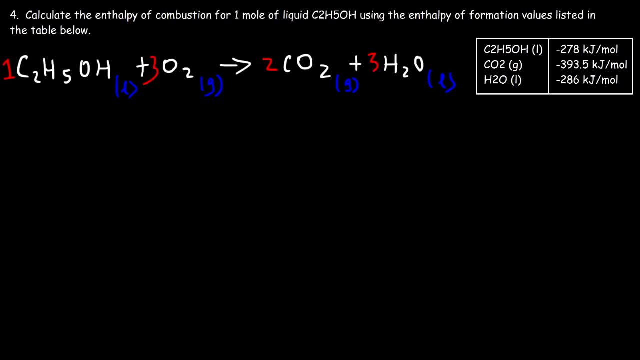 of O2.. And now the chemical reaction is balanced. So now let's calculate the enthalpy change. Because this is a combustion reaction, the enthalpy change of this reaction is equal to the enthalpy of the combustion. So the finite enthalpy of combustion from 1 mol of ethanol. we just need to find the. 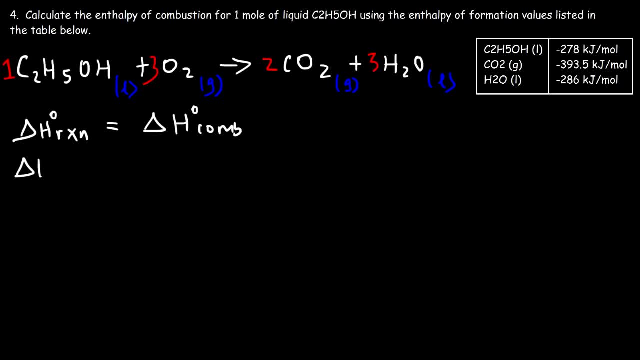 enthalpy of that reaction. And we can calculate the enthalpy change of the reaction using the same technique as what we did before: products minus reactants. So it's going to be the sum of all the heat of formation of all the products. 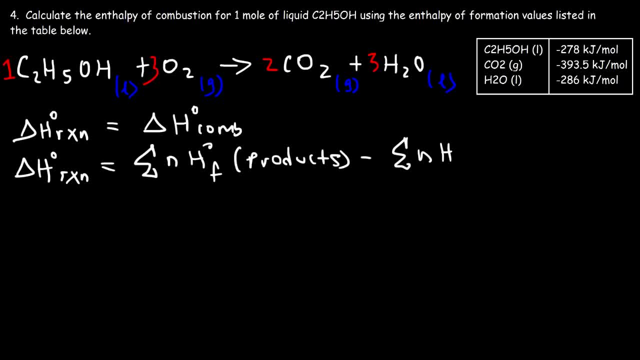 Minus the sum of the heat deformation of all the reactants. So these are the products. You can find it on the right side, So that's 2CO2 plus 3H2O, And the reactants on the left side. 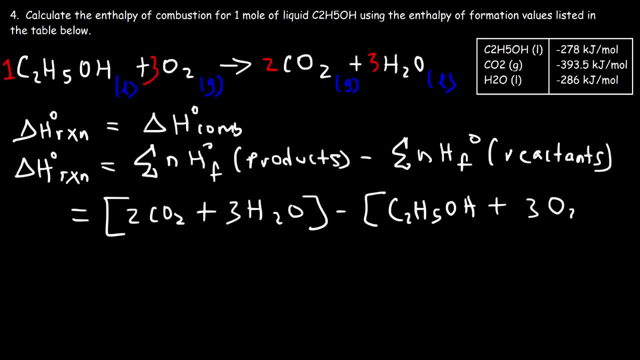 C2H5OH plus 3O2.. So now let's plug in the values that we have. So the heat of formation for carbon dioxide is negative 393.5.. And the enthalpy of formation for liquid water is negative 286.. 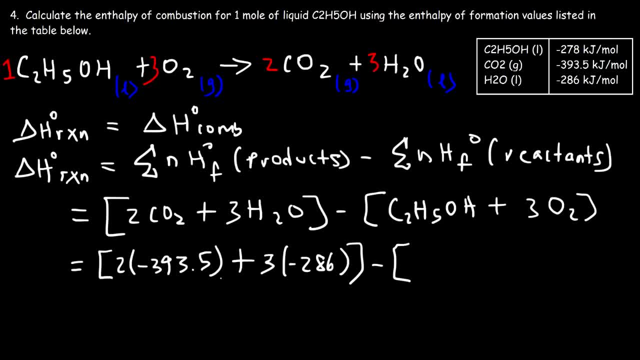 The enthalpy of formation for ethanol is negative 278.. And O2 is a pure element in its natural state, so it's going to be zero. So let's go ahead and plug these numbers in. So I got negative 1367 kilojoules per mole. 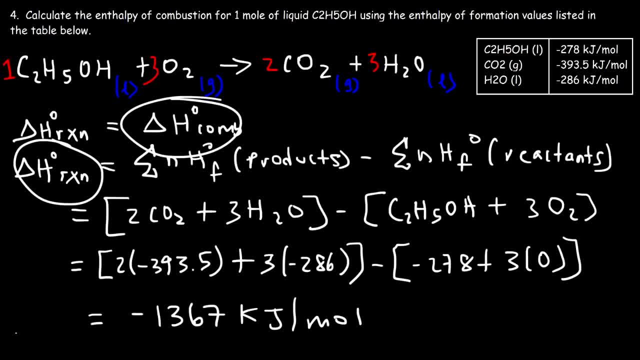 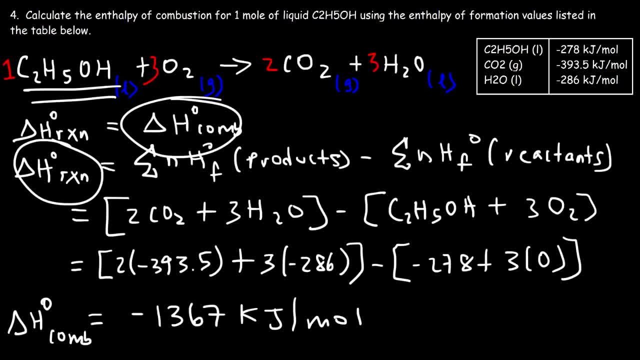 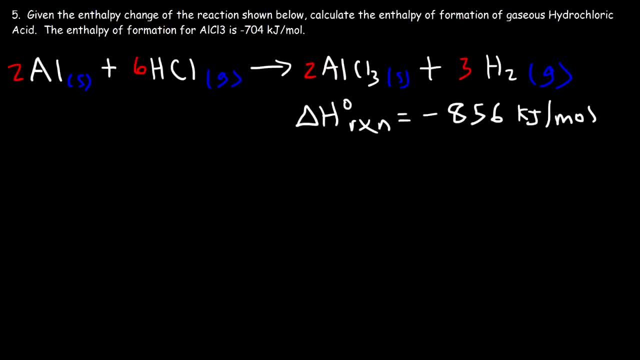 For the reaction For one mole of C2H5OH, also known as ethanol. Now let's move on to our last question. Given the enthalpy change of the reaction shown below, which is negative 856 kilojoules per mole, 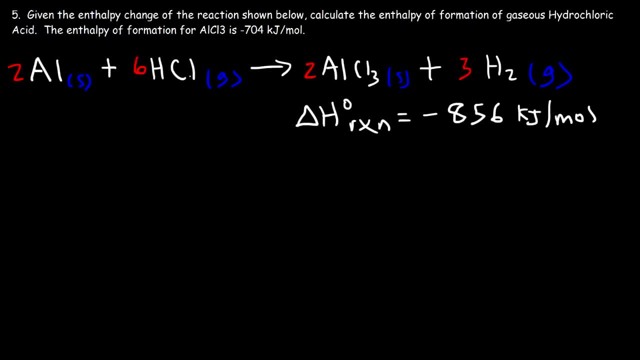 Calculate the enthalpy of formation of gaseous hydrochloric acid And we're given the enthalpy of formation for AlCl3.. AlCl3. Which is negative, 704 kilojoules per mole. So how can we calculate the enthalpy of formation for HCl? 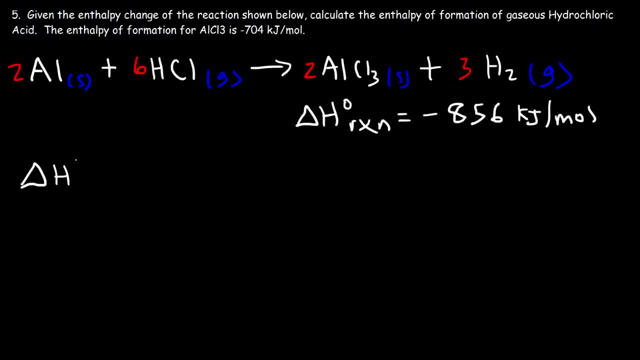 Well, let's start with the equation. We know that the enthalpy change of the reaction is going to equal the sum of the heat of formation of the products, which are those two: aluminum chloride and hydrogen gas. Don't forget to take the coefficient. 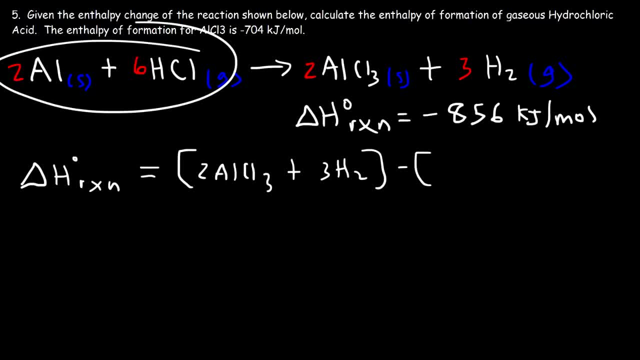 into account minus the sum of the heat of formation of the reactants, which are aluminum and hydrochloric acid. So all you need to do in this problem is you need to plug in all the values that you have and simply find the missing value. 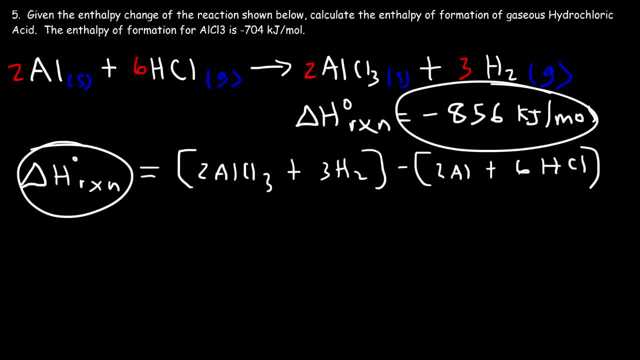 We have the enthalpy change of the reaction: it's negative 856, so we got that. Now we have the value for AlCl: It's negative 704, so we got that as well. Now what's the value for hydrogen gas? because we didn't receive that value. it. 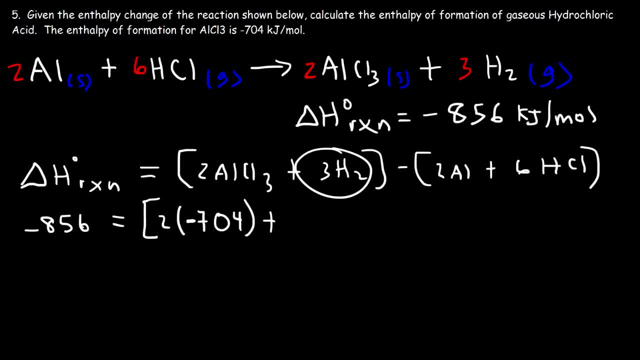 was not given to us in this problem. Now, this is a pure element in it's natural state, so it's zero. That's why it wasn't given to us. Aluminum is also a pure element in it's natural state, so the heat of formation for aluminum is zero. 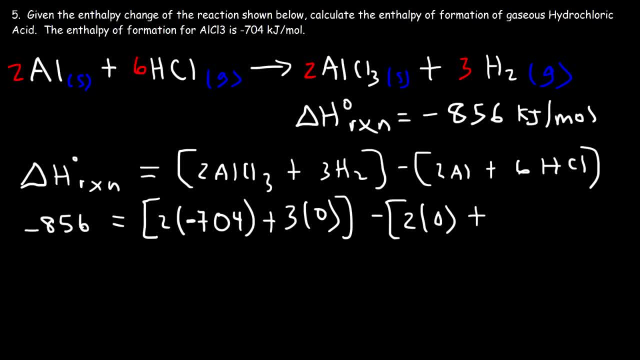 So now we need to solve for HDL, So I'm going to put an x in place of HDL. So our goal is to calculate x. So first let's multiply negative 704 by 2. And so you should get negative 1408.. 3 times 0 is 0, and 2 times 0 is 0, so you could just ignore those values.